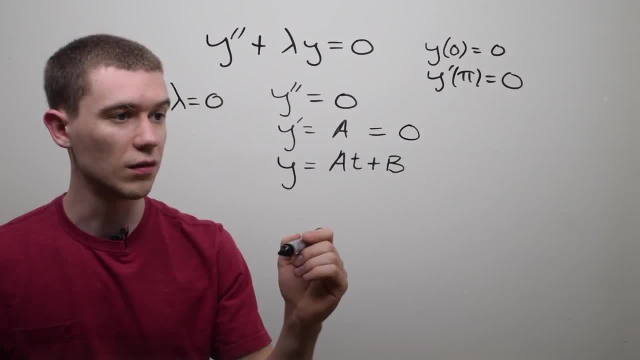 for pi. So this is just equals zero. So, in other words, a is equal to zero. it's kind of boring. well, that means this whole term is going to drop out, right? And I can use the same logic with this first condition that y of zero is equal to zero. Well, that means I plug in zero for y. 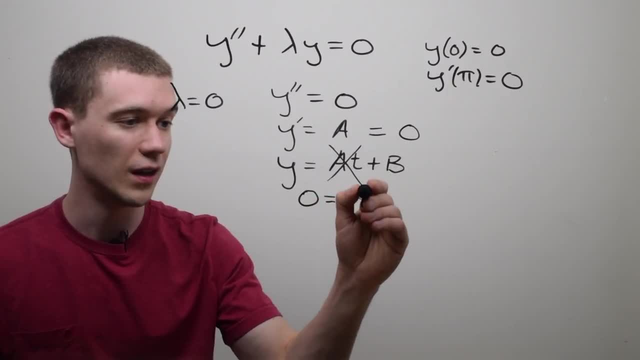 plug in zero for t. well, there's nothing really to plug in anymore. I'm just getting that b is equal to zero. Well, if a and b are zero in this equation, that means I just have y is equal to zero, And in other words, I've got a trivial solution, And that's pretty boring. 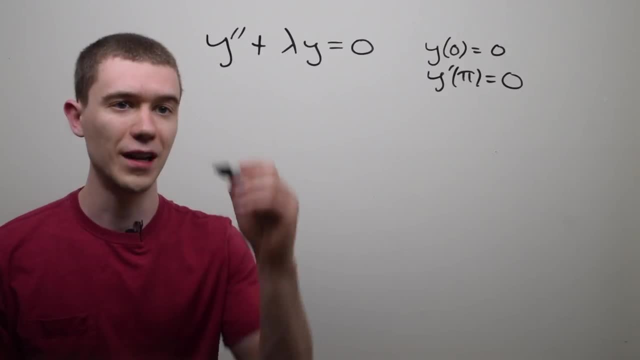 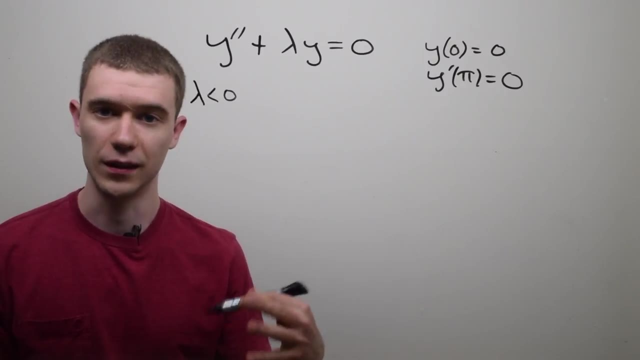 If lambda zero, we get a trivial solution. What about if lambda is negative? Well, if lambda is negative, all of a sudden this becomes something I can solve using the techniques you've probably learned earlier in your differential equations class. So I would reduce. 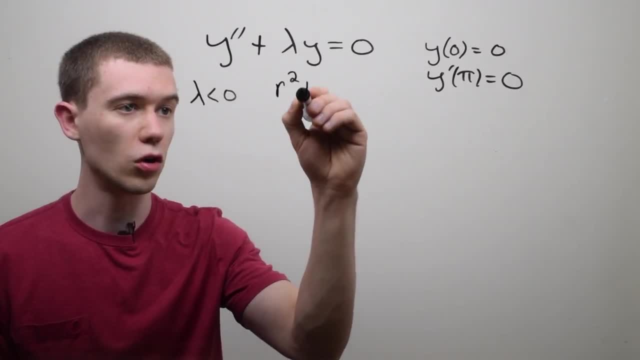 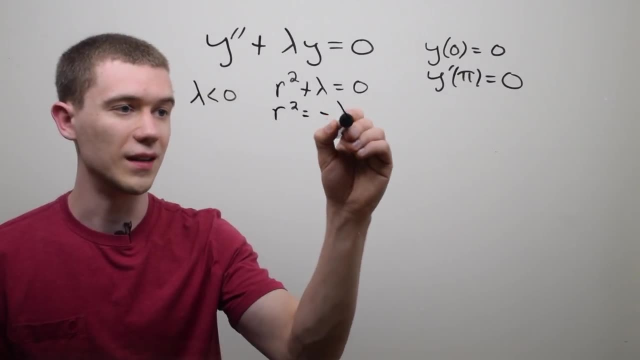 this to the auxiliary or characteristic equation: r squared plus lambda is equal to zero, And this means that r squared is equal to minus lambda, or that r is equal to plus or minus square root of minus lambda. Now this might look a little weird, But remember, lambda is negative. So this is: 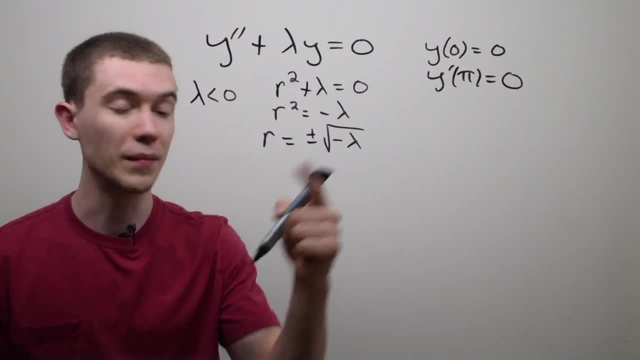 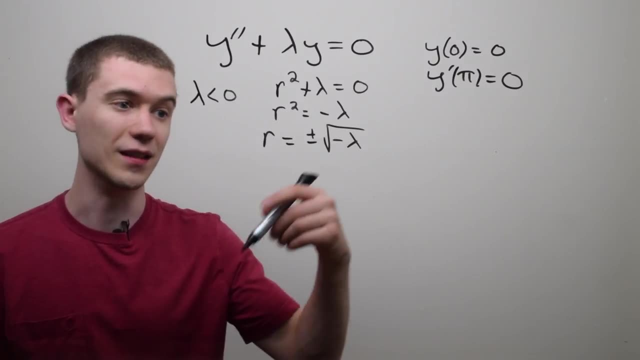 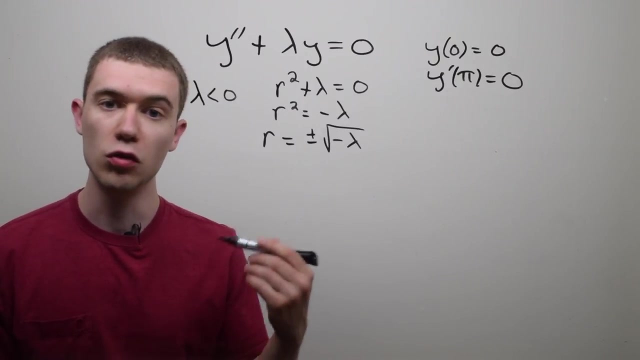 really a positive inside the square root. In other words, I'm getting two real roots, one being plus root, lambda, and one being minus root, lambda, minus root, minus lambda. that is So. if you have two roots of the auxiliary or characteristic equation, what's your solution? Well, it has the form y equals c, one e to the 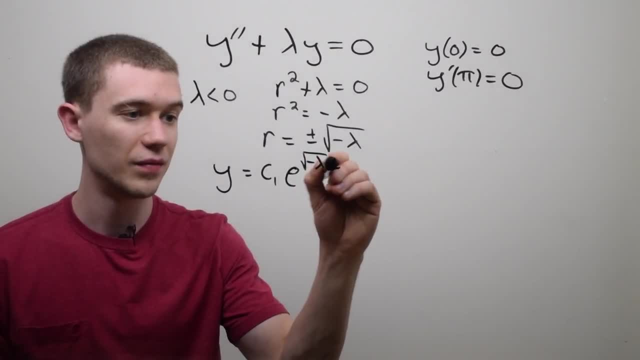 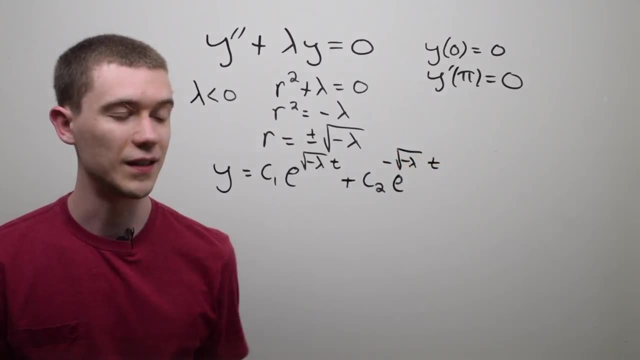 first root, so that's root minus lambda t plus c, two e to the other root, That's minus root minus lambda t, And I can use these initial conditions again. So the first one says that if y of 0 is 0.. 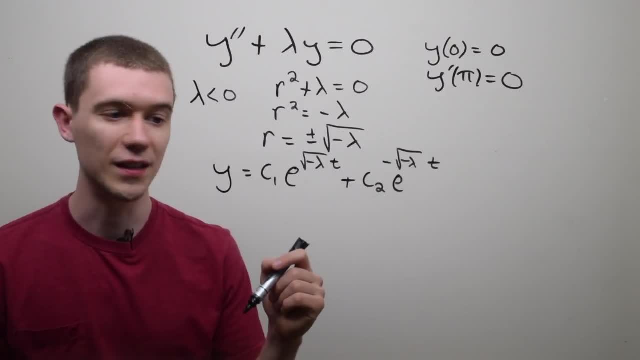 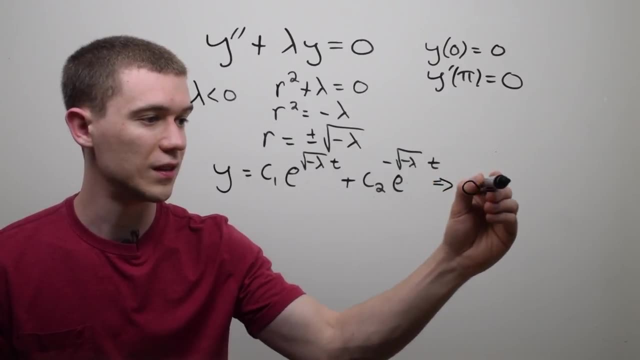 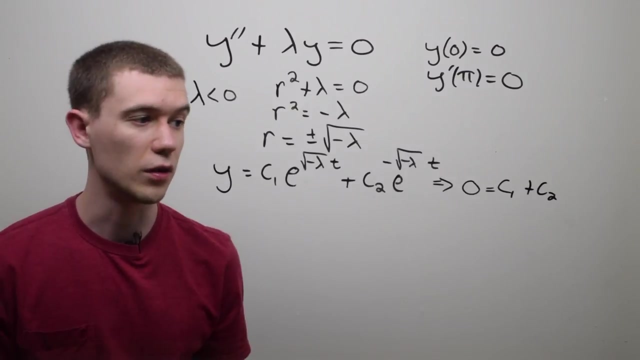 So in other words, if I plug in 0 for t, I should get 0 for y. Well, that's going to mean that 0 is equal to c1.. e to the 0 is 1, plus c2, e to the 0 is 1.. 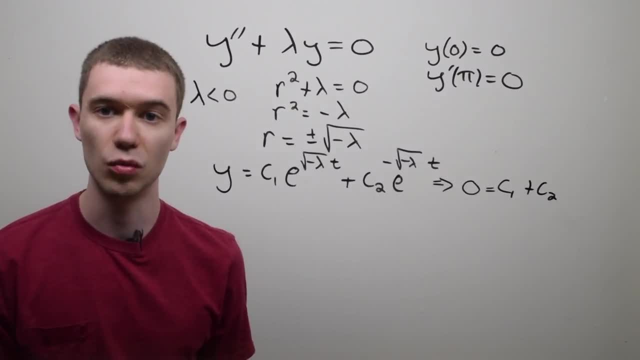 OK, I've got one equation And I'm going to need to take the derivative in order to get this second equation, So let's just take the derivative here real quick. And so that comes from just using differentiation rules on the exponential function. 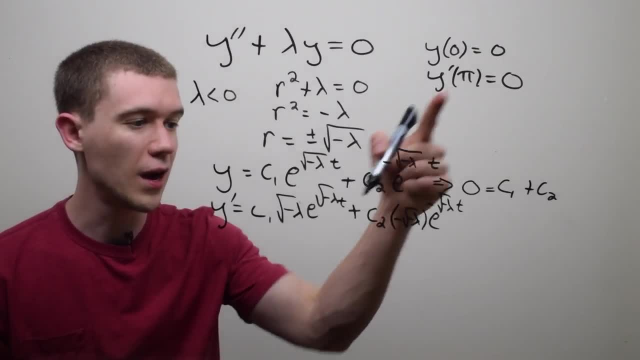 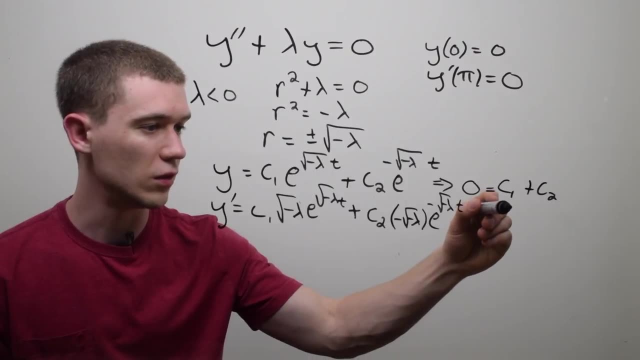 Now, if you'll notice from this initial condition, if I plug in pi for t, I should get 0 for y. Before I'm going to do that, I'm going to go over here. Notice that c1 plus c2 is 0.. 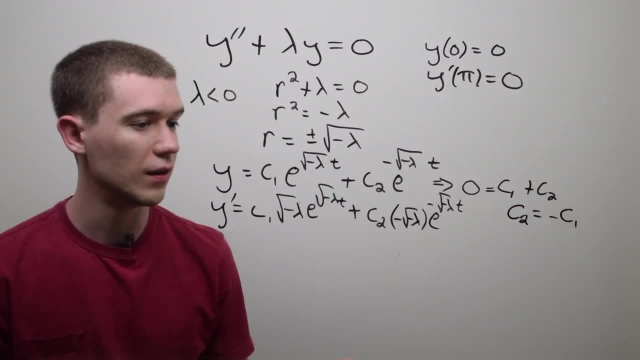 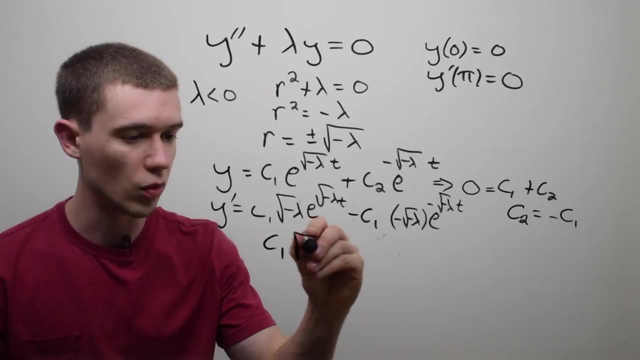 That means c2 is equal to minus Minus c1. So I could just replace this c2 with minus c1. And what I'm going to do is I'm going to factor out that c1. And I'm going to factor out that square root of minus lambda. 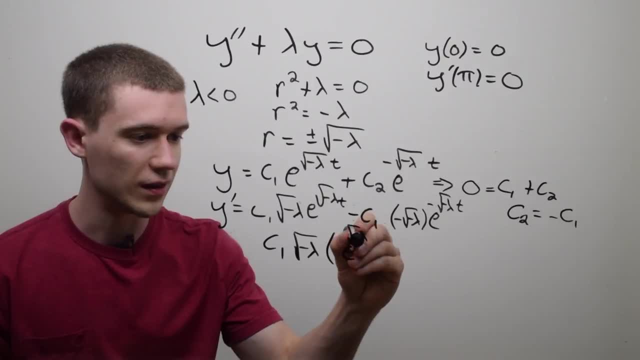 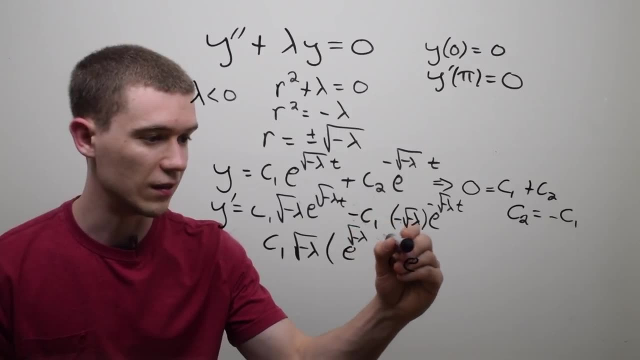 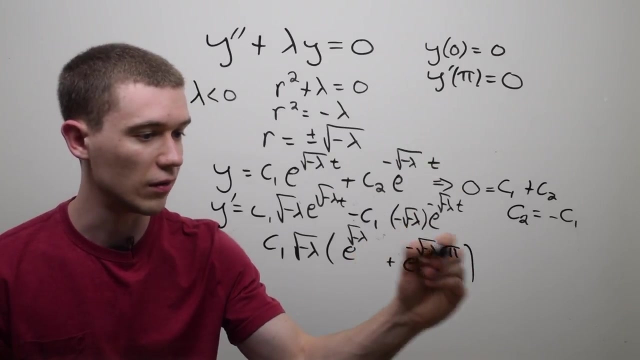 And that's just going to give me e to the root minus lambda, t minus minus a minus, So it's going to be a plus e to the minus square root minus lambda And that's going to give me 0 for t. And this initial condition says that if I plug in pi for t, 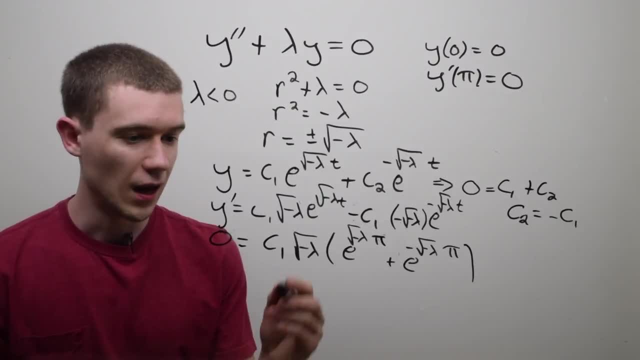 that's going to give me 0.. Well, take a look at this. Minus lambda, square rooted, is not 0. We assumed that because lambda was negative, I've got e to something plus e to something else. So this piece is not equal to zero. this piece is not equal to zero, but I have things. 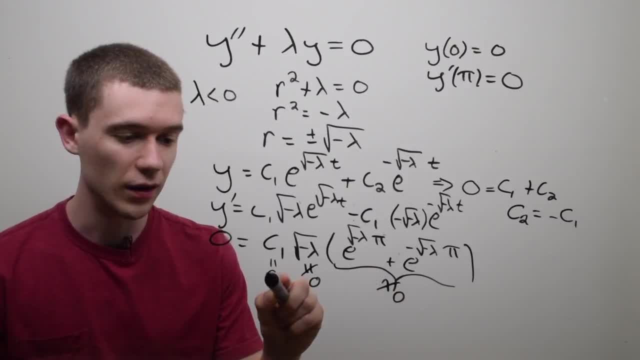 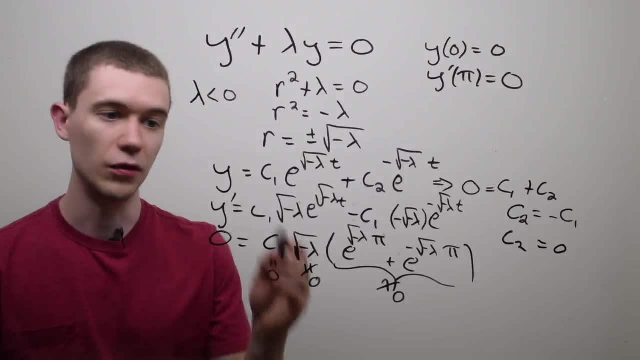 multiplied equal to zero, That means that c1 has to be zero. And if c1 is equal to zero, that means c2 is equal to zero. And if you go to our y equals equation, that means I've got y equals zero and plus zero. 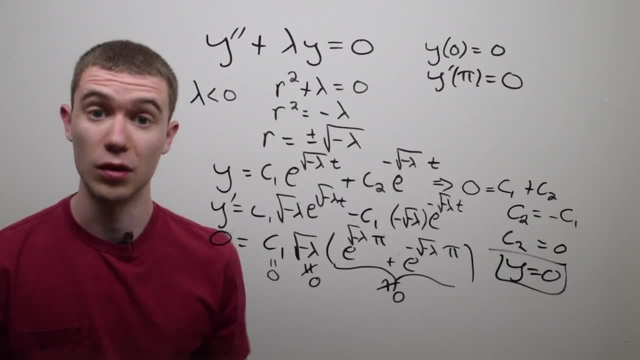 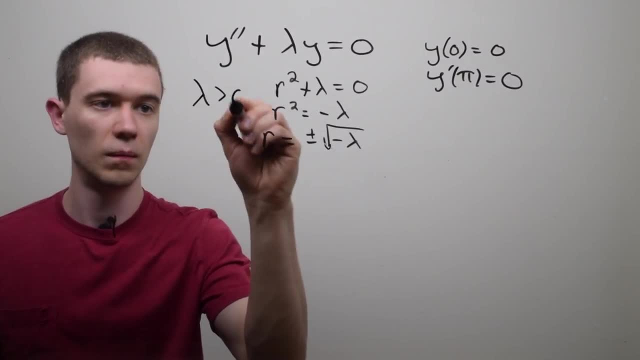 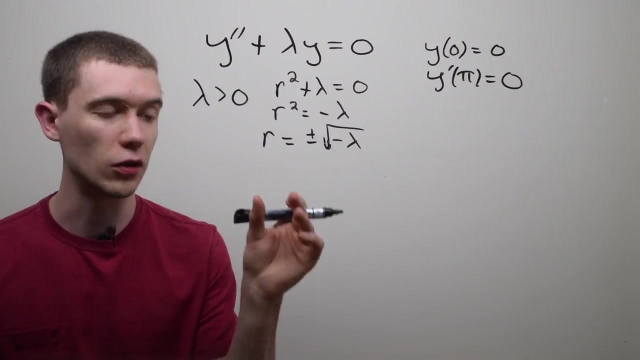 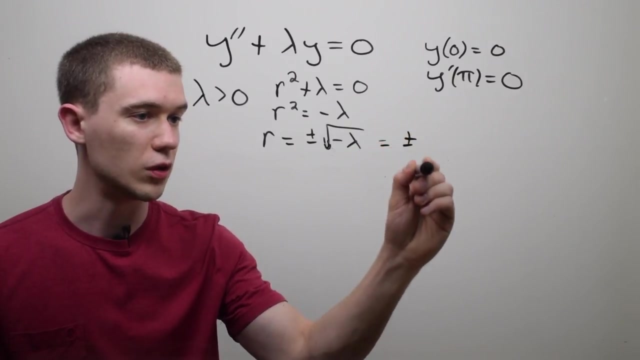 So, in other words, I have the trivial solution once again. Now things finally start to get interesting when lambda is positive, because although the roots of the characteristic or auxiliary equation are the same, since lambda is positive this is actually a negative under the square root, which means these values are really 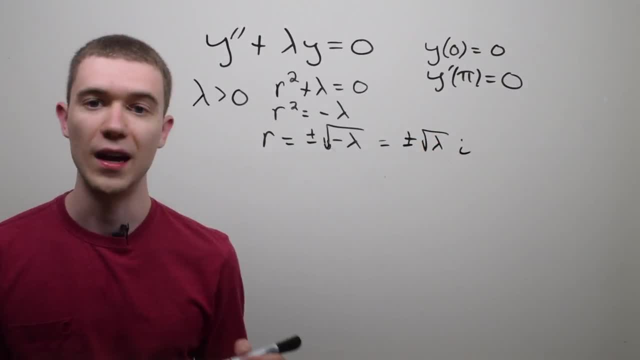 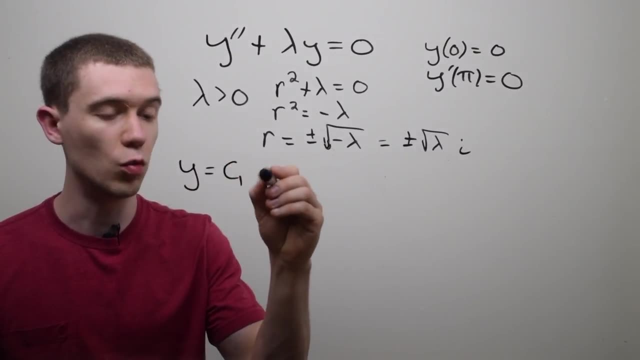 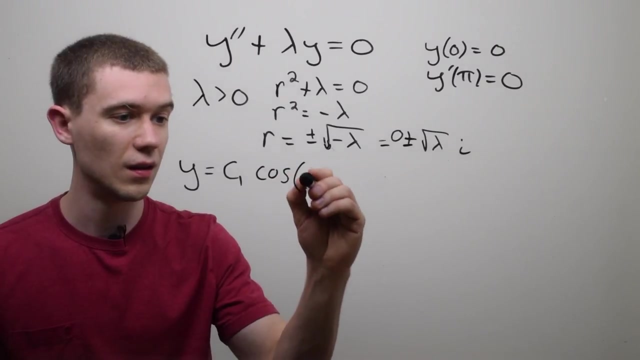 plus or minus square root of lambda i. And when you have imaginary roots to your characteristic or auxiliary equation, the solution looks like this: Y equals c1, e to the real root, in other words, e to the zero cosine of the imaginary part. 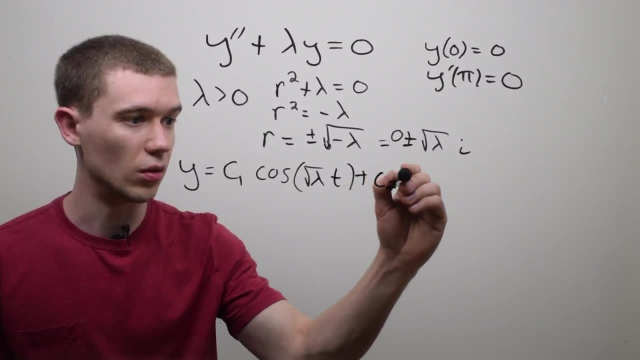 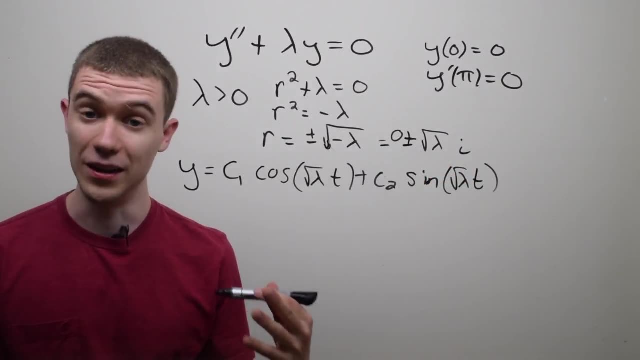 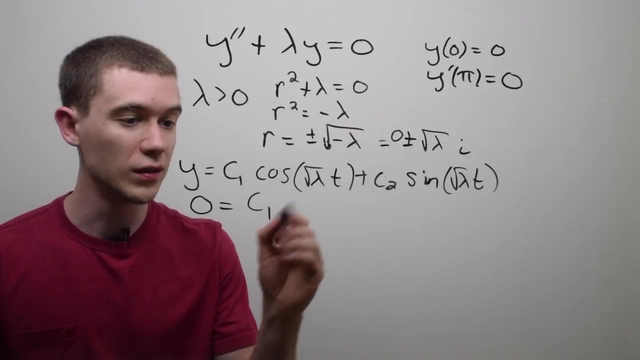 t plus c2 e to the zero sine, the imaginary part times t. Now let's use our initial conditions again: Y of zero is zero. That means I'm going to get zero for y. This would be: c1 cosine of zero is one plus c2 sine of zero is zero. 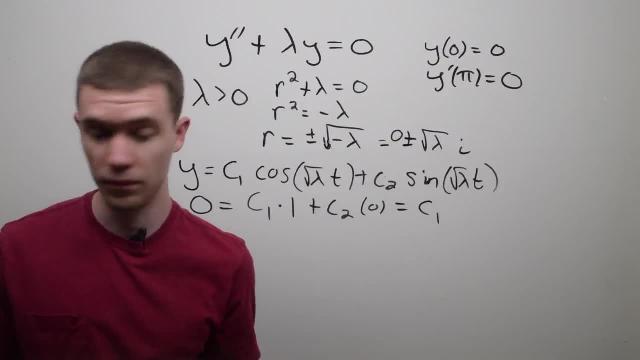 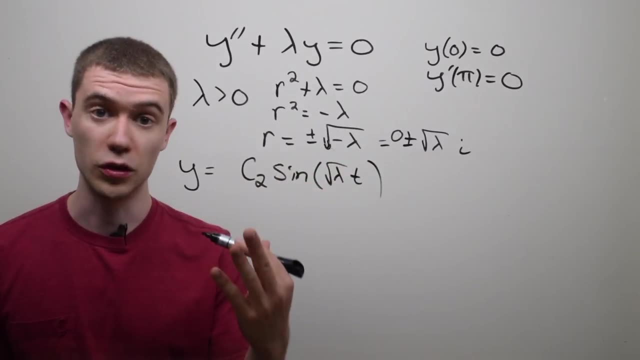 So it looks like I'm getting. c1 is equal to zero, So our solution reduces to just c2, sine, square root lambda t. To use this other initial condition, I'm going to have to take the derivative. So that's just taking the derivative of sine. 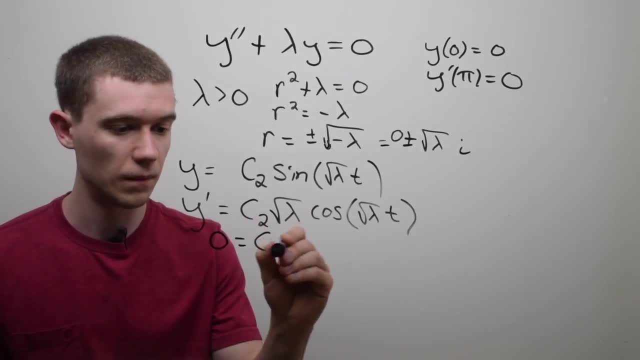 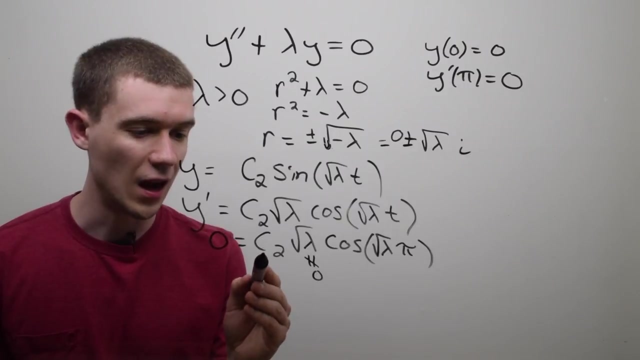 And if I plug in pi, I'm supposed to get zero. Now let's observe something again: Square root lambda is not equal to zero. by assumption, Lambda is positive, I'm also going to assume now that c2 is not equal to zero. 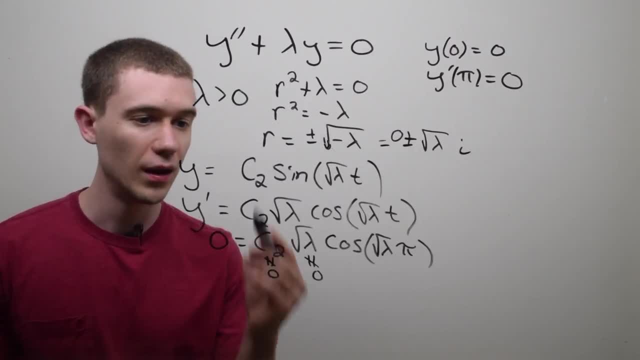 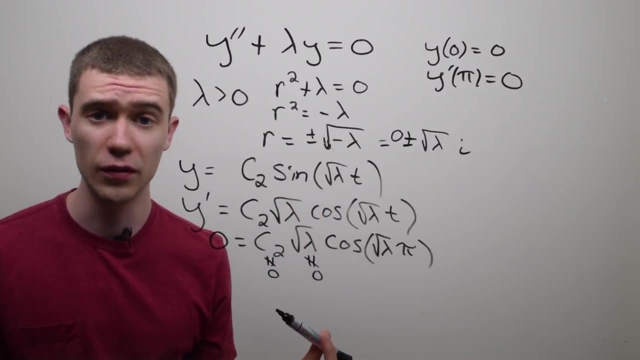 Now why is that? If c2 was zero, well, I'd have y equals zero. I'd have the trivial solution again, And that means, no matter what lambda was, I'd have the trivial solution. Now I want to get something from this, so I'm going to say c2 is not zero. 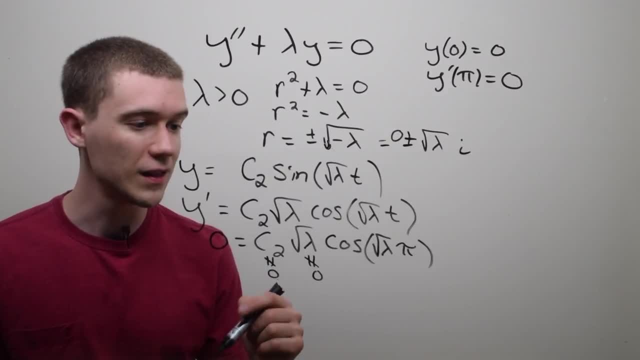 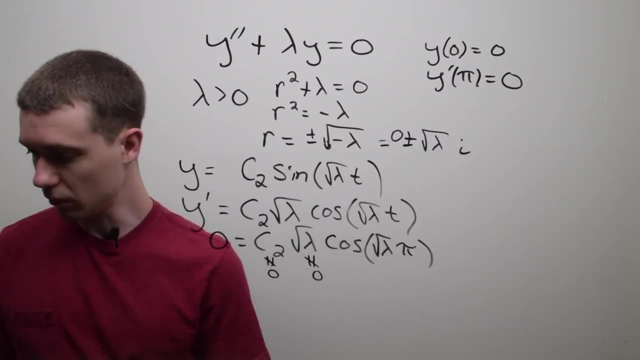 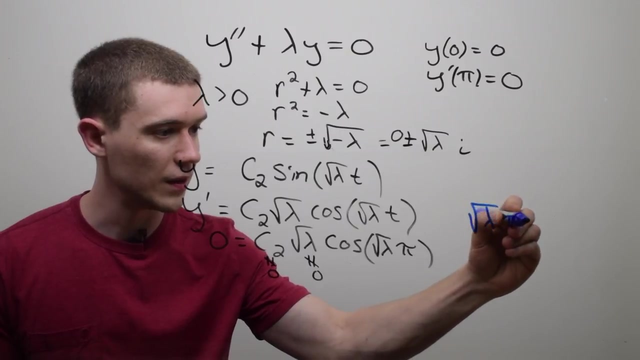 Well, if I have things multiplied being zero, that must mean that this cosine factor has to be zero. Now, when is cosine zero? Cosine is zero When the inside, When the outside, is equal to an odd multiple of pi over two. right? 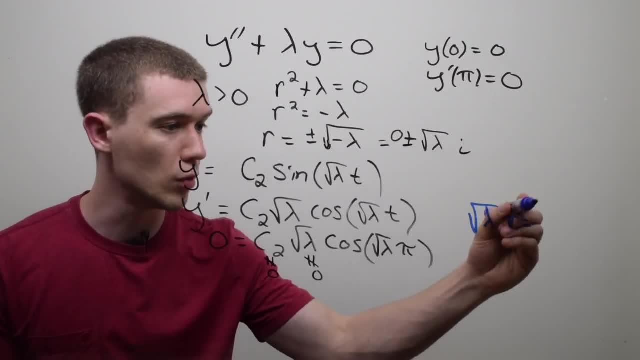 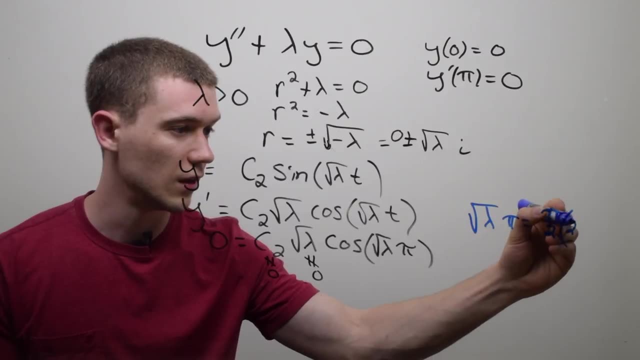 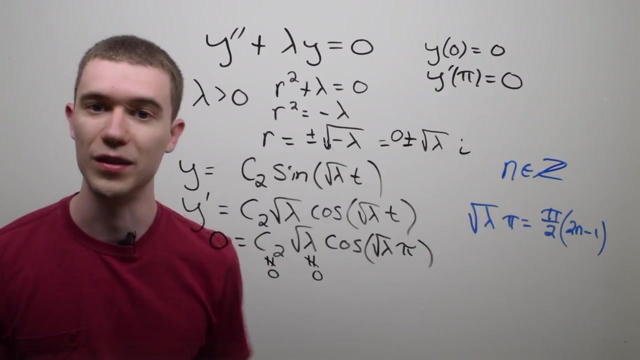 Pi over two, three pi over two, five pi over two And the way we represent that is pi over two times some odd number And an odd number looks like. I'll say 2n minus one And you can check that for n in the integers is how we say that.